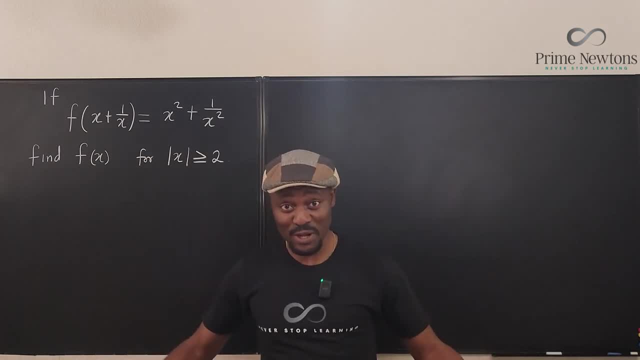 I know there are many people who watch these videos, who do a lot of math and try to prove all the things that are necessary. Let's just get what f of x is Okay, Um, so the first thing I'm going to do is- I've seen this before because I know that you can generate. 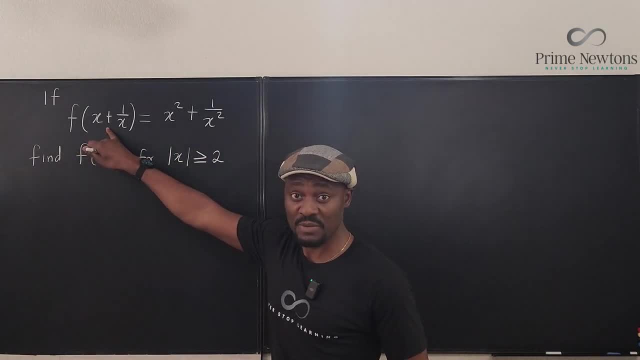 this from a problem. I know that you can generate this from a problem. I know that you can generate this by squaring this argument. so what I'm going to do is here I'm going to say that consider X plus 1 over X squared. I just want to see, because what I'm trying 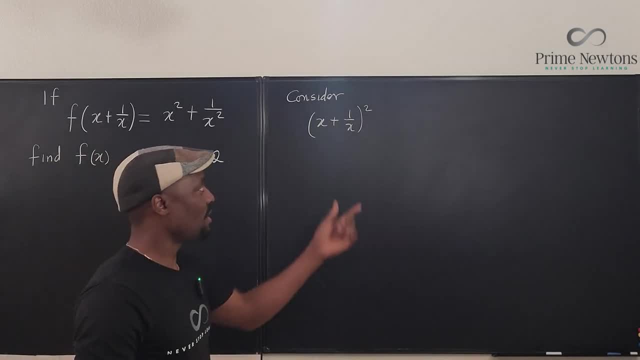 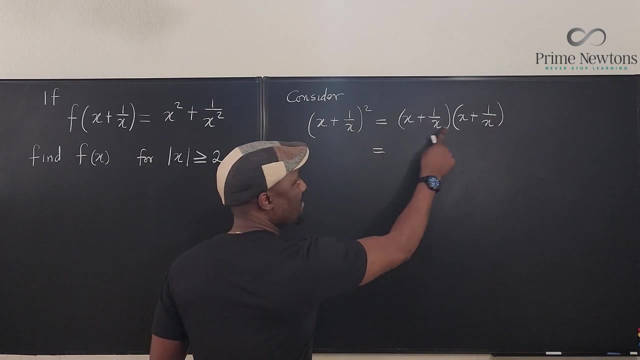 to do is: I'm trying to create this. okay, I want to see if I can create it from here. this is the same thing as X plus 1 over X times X plus 1 over X. you notice that if I distribute this, I'm going to end up with X squared plus X times 1. 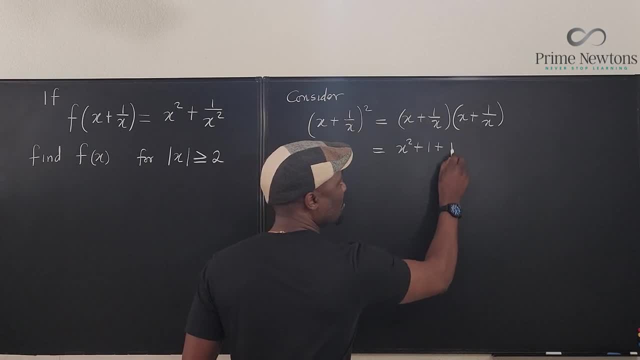 over X is 1. this times this is 1 and this is 1 over X squared. so, as you can see, I have X squared plus 1 over X squared, plus 1 over X squared. so, as you can see, I have X squared plus 1 over X. 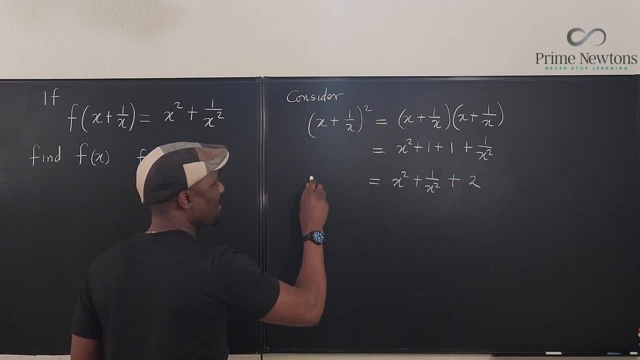 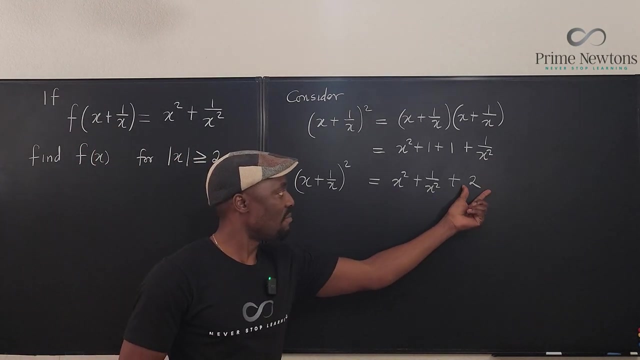 squared plus 2. that's what I have on this side: X plus 1 over X, all squared. so it means, if I go back to this function, I could actually say that F of X plus 1 over X is this. well, let me just isolate this by moving this here, so I can say: 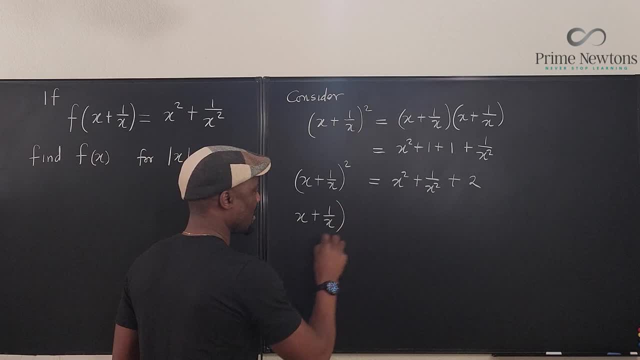 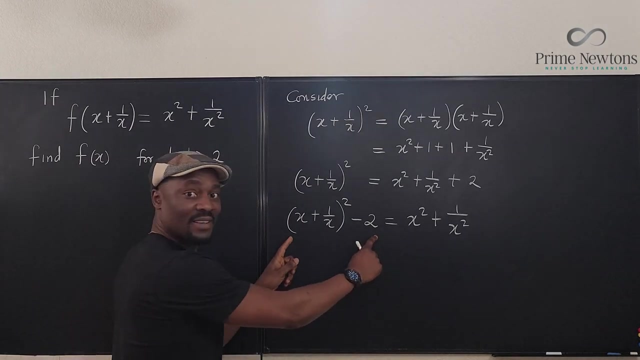 that X plus 1 over X squared minus 2 is equal to X squared plus 1 over X squared. I just move this over here. that means when the argument is X plus 1 over X, the output is 1 plus 1 over X squared minus 2. that is this. so I can say F of X plus 1 over X, which is: 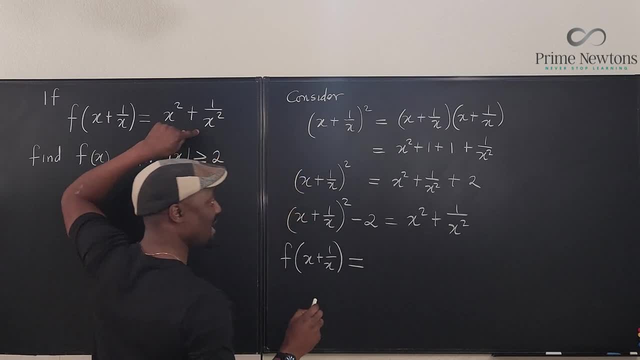 what we have here is equal to this, but this is represented as this, which is x plus 1 over x squared minus 2. so that means I can clearly say that when you give something to F, what does it do with it? it squares it and then subtracts 2. 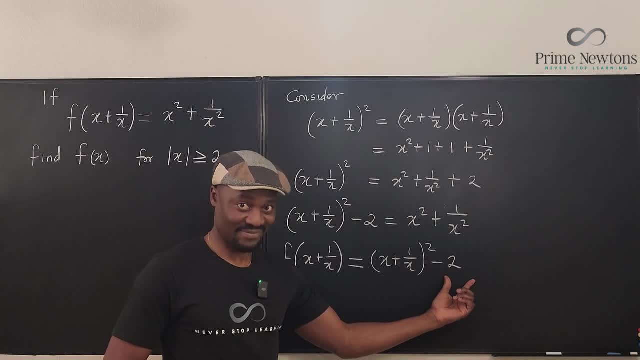 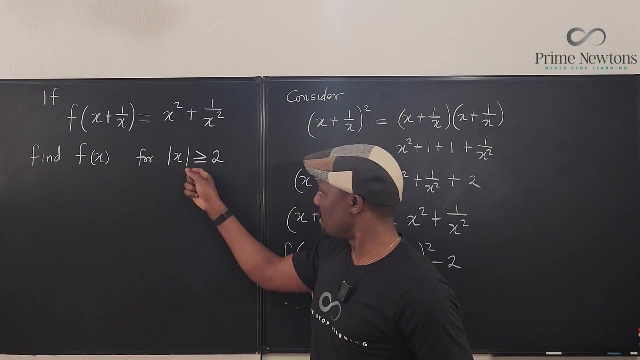 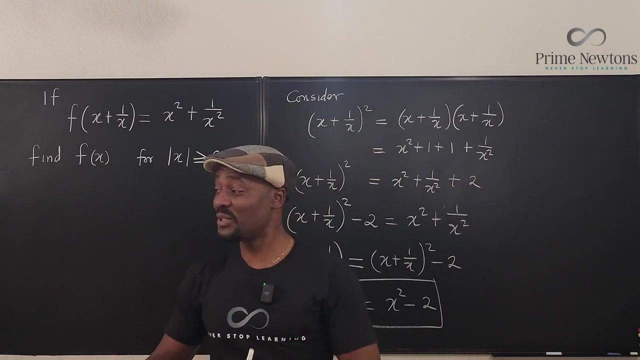 from it. so I can say: therefore, f of X is equal to x squared minus 2. this is the function. now, why does it have to be this? well, this is necessary because if you had done the T substitution replacing this, there's going to be a problem on. 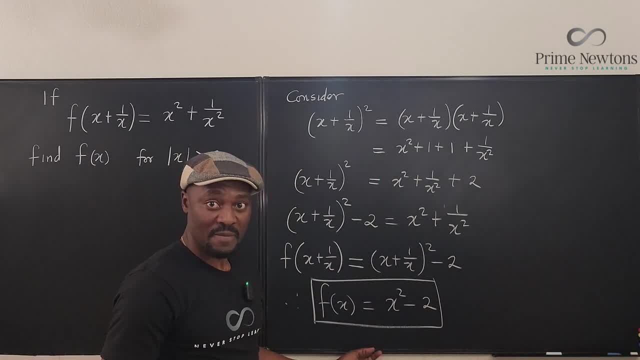 the way, not everybody would have done it. well, this is necessary because if you had done the T substitution replacing this, there's going to be a problem on the way. not everybody would have done it this way. in order to make that valid, let's just see what happens if we try to. 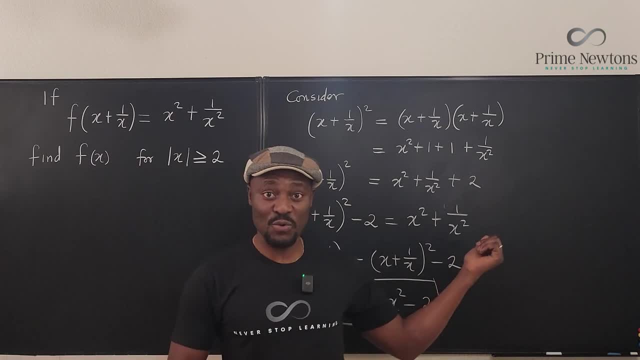 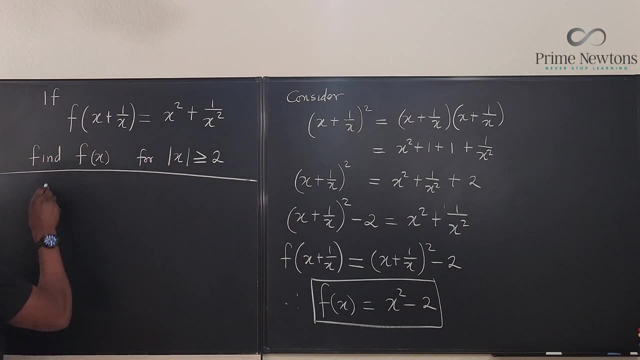 do a T substitution and try to isolate X to go replace there. it's more complicated, so let's see. so let's say: let T be equal to X plus 1 over X. from here, it simply means that T minus X equals 1 over X. T X minus X squared equals 1. you can form a quadratic equation from here and: 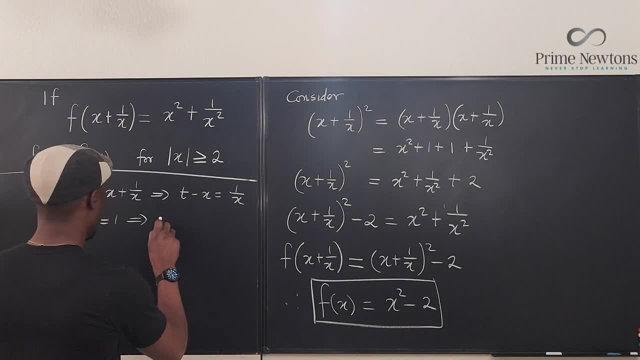 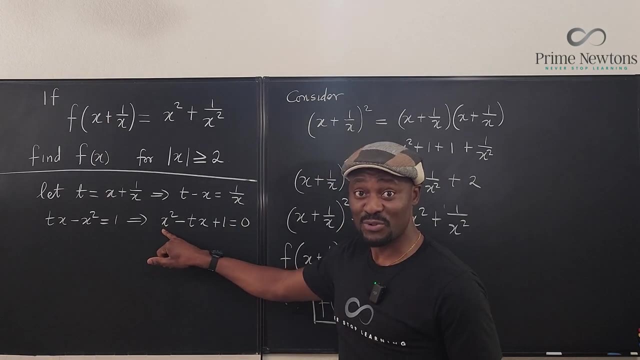 that gives us. what do we have? we're going to get X squared minus T. X plus 1 is equal to 0, so you will need to solve a quadratic equation to get what X is because, remember, we have to write X in terms of T, and that is where the 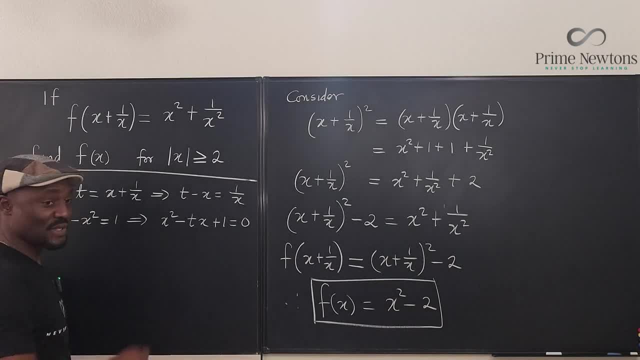 square root of X is. so you use the quadratic formula because this cannot be factored. we don't know what T is, so we can say that X equals minus B plus or minus square root of B squared. so we say a minus B is just going to be T plus, or.